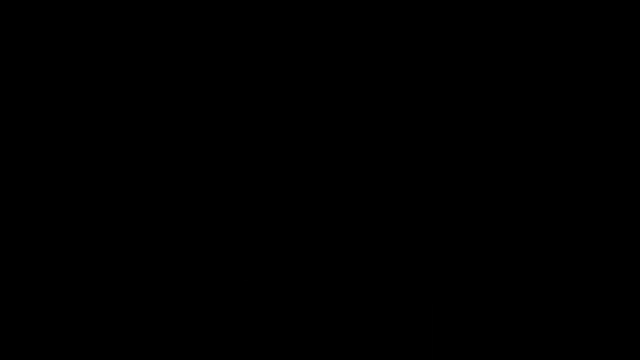 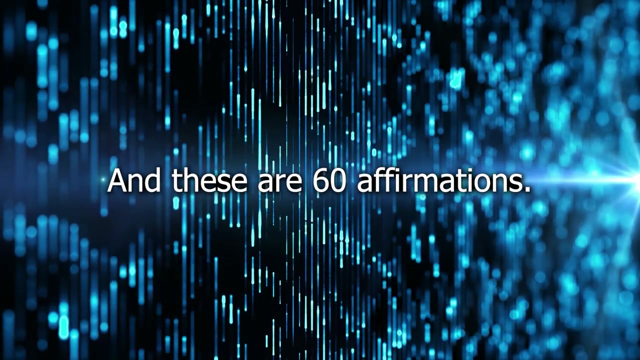 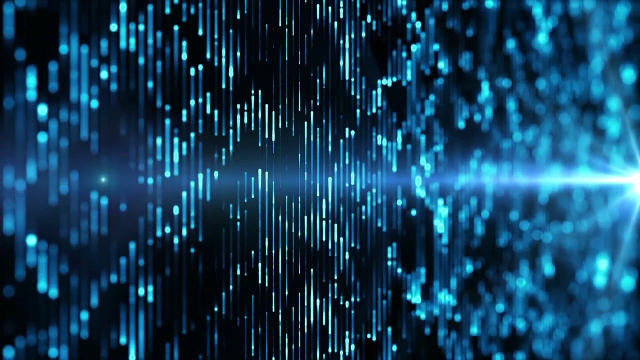 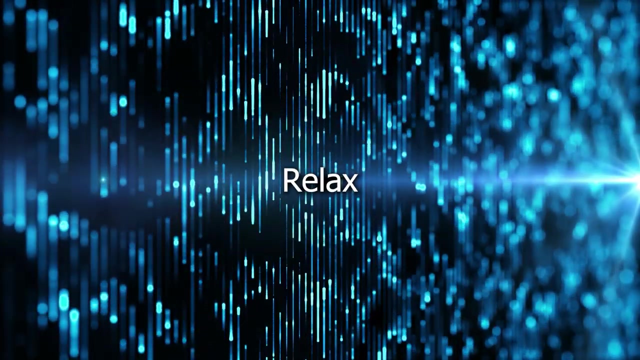 Hi, this is Dare To Do, Motivation, and these are 60 affirmations for those of you who are constantly overthinking, are anxious and have too much noise in their mind. So sit down, close your eyes, relax and listen to these affirmations. 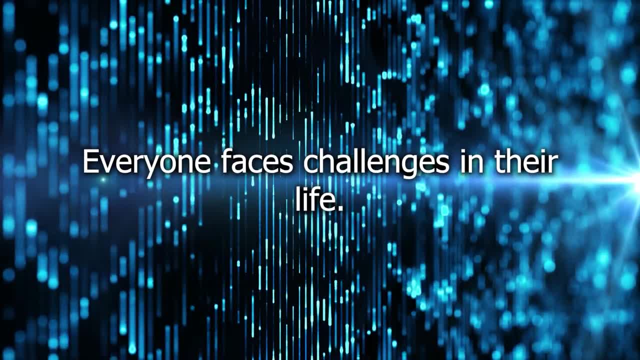 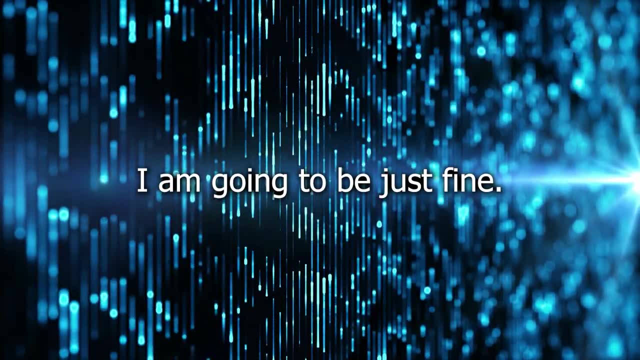 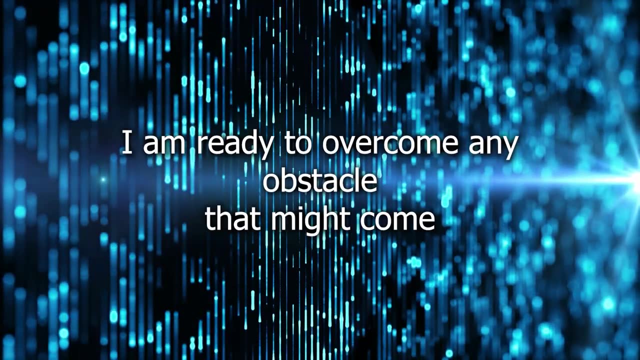 Everyone faces challenges in their life. I am going to be just fine. I have been through this before and I have survived. I am ready to overcome any obstacle that might come my way. I am ready to overcome any obstacle that might come my way. 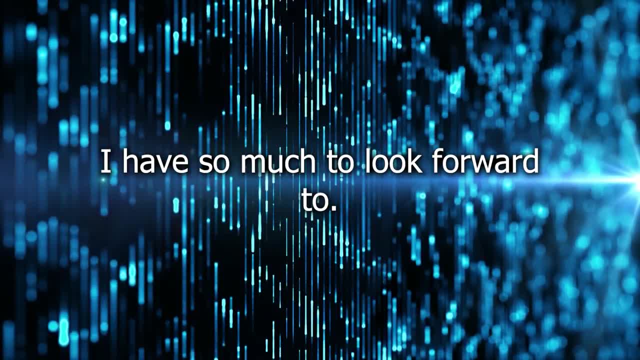 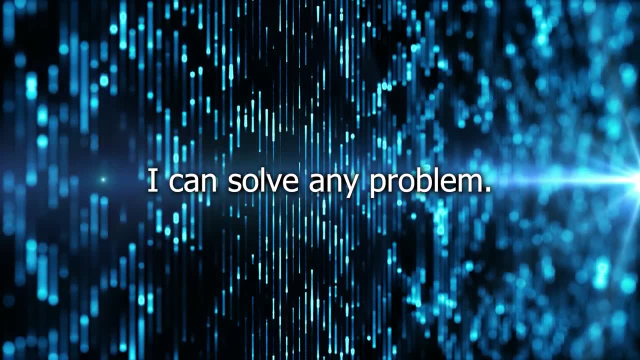 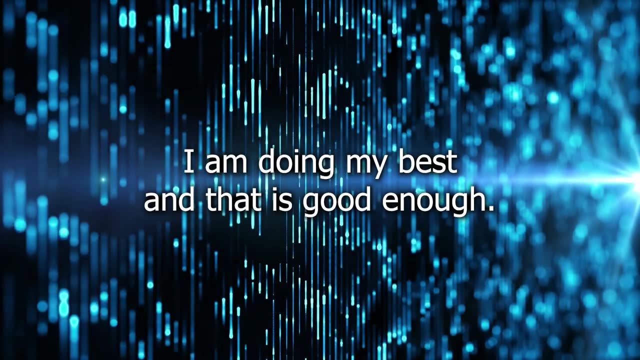 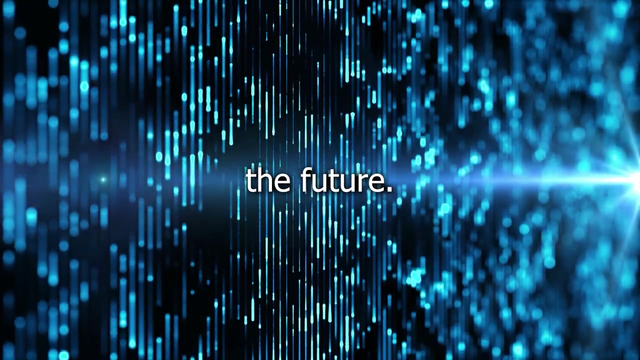 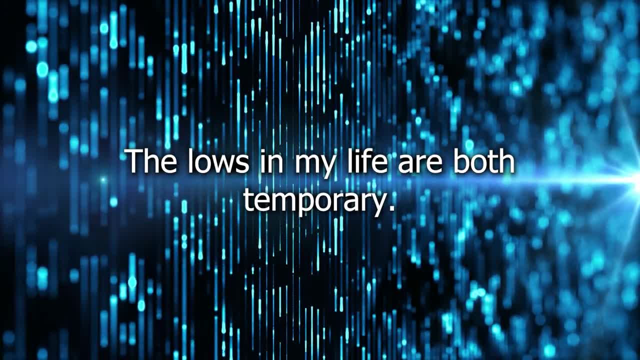 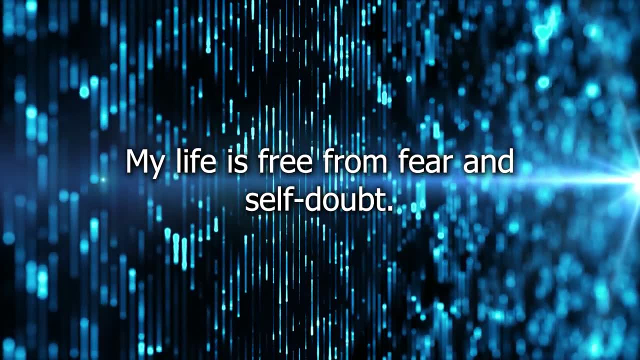 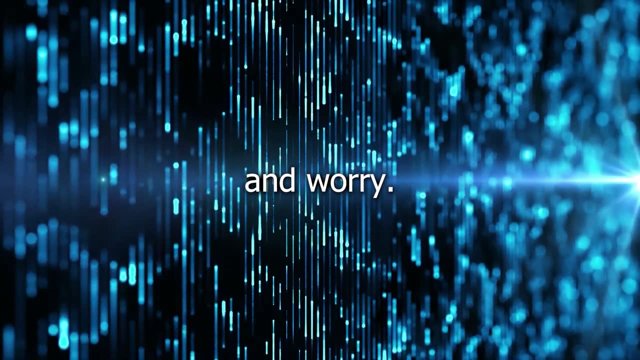 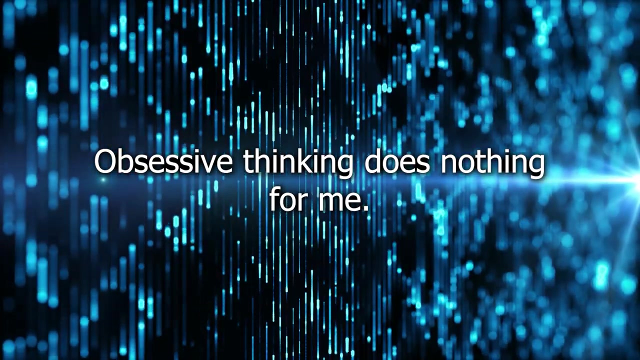 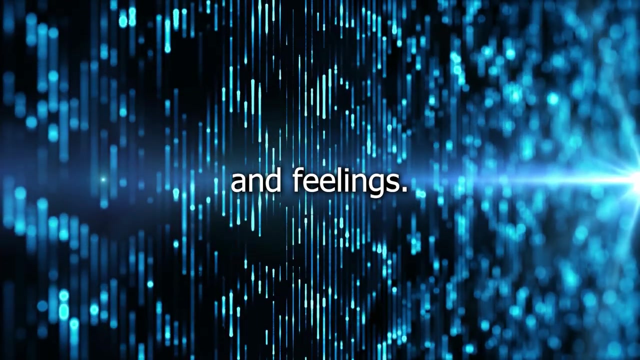 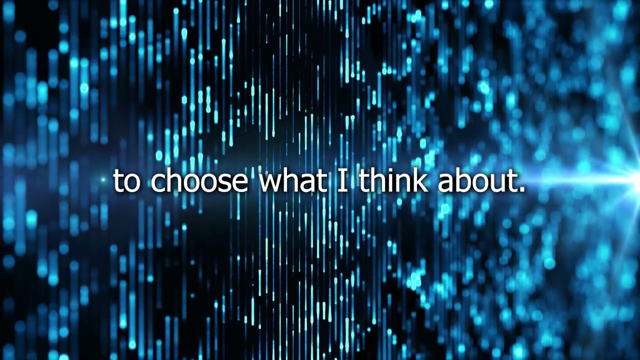 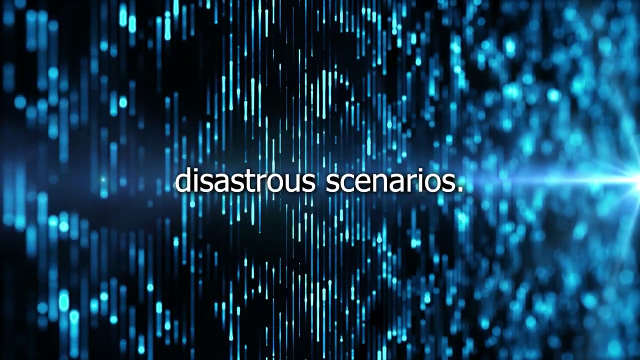 in my life are but temporary. My life is free from fear and self-doubt. I am free from anxiety and worry. Obsessive thinking does nothing for me. I am in complete control of my thoughts and feelings. I have the power to choose what I think about. I refuse to let my imagination create disastrous. 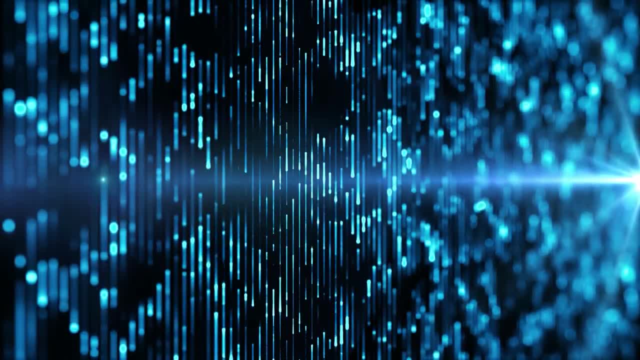 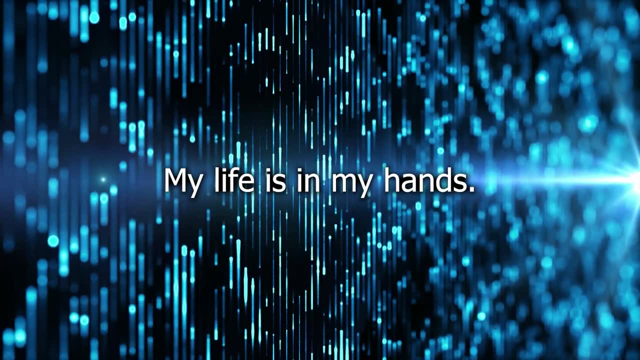 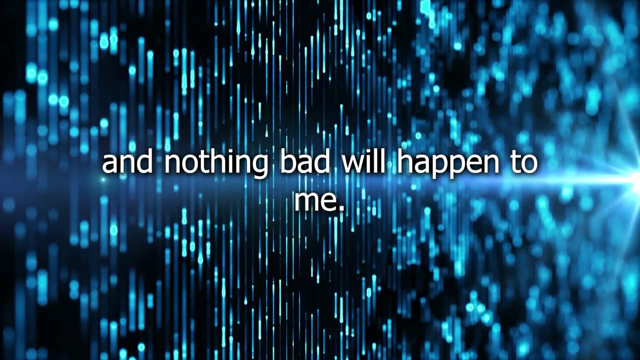 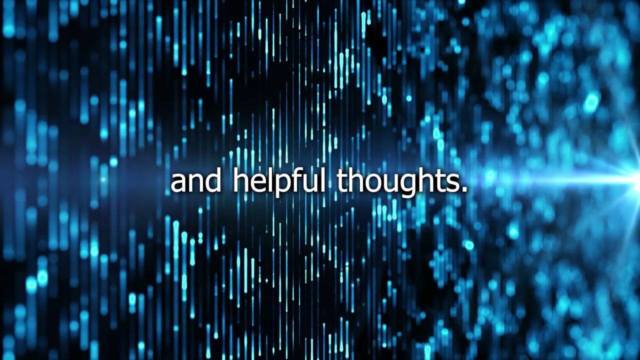 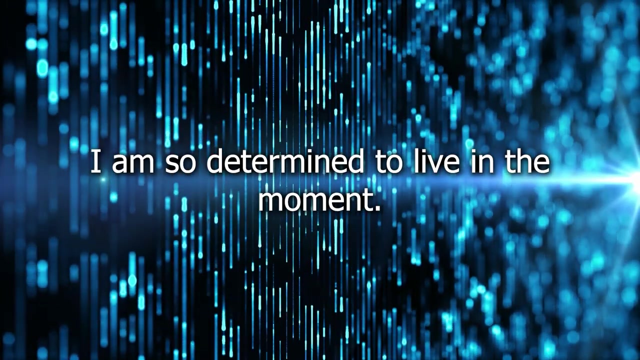 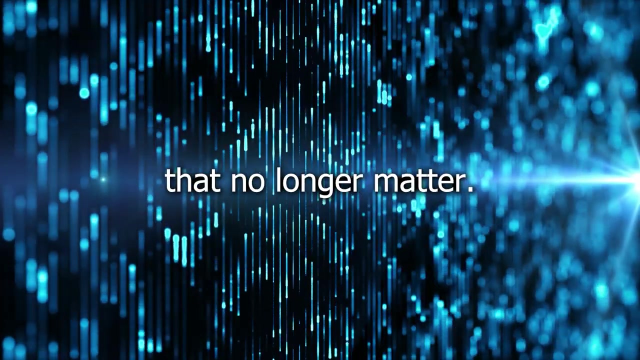 scenarios. I am in charge of my mind. My life is in my hands, I am safe and nothing bad will happen to me. I choose to focus on the positive and helpful thoughts. I am so determined to live in the moment. I can let go of things that make me feel more. 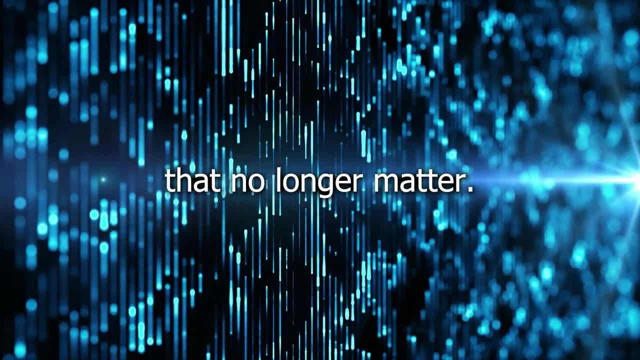 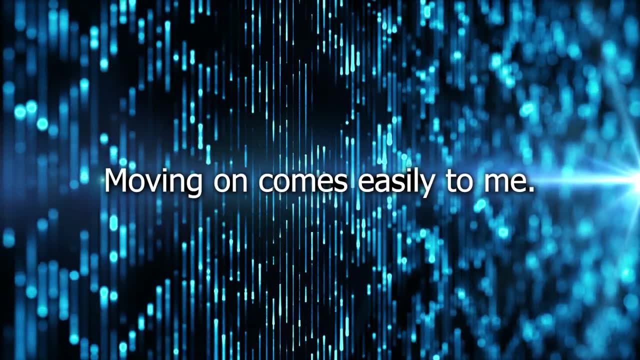 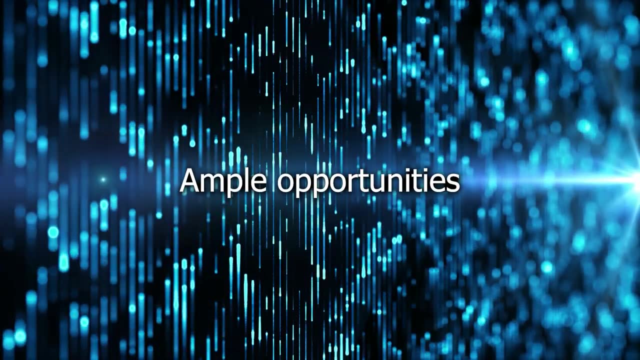 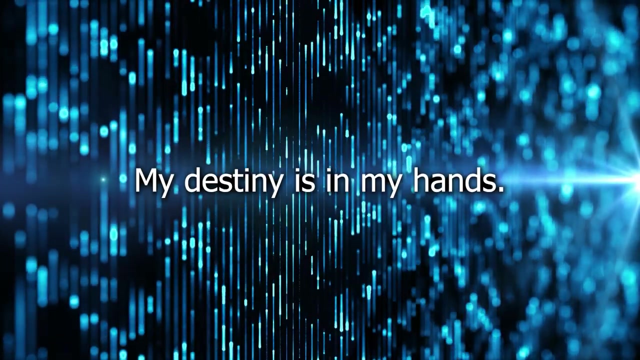 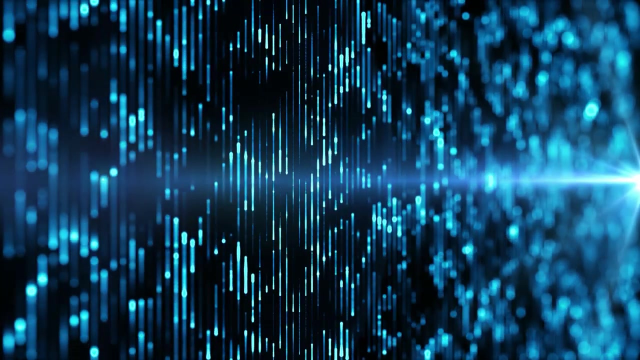 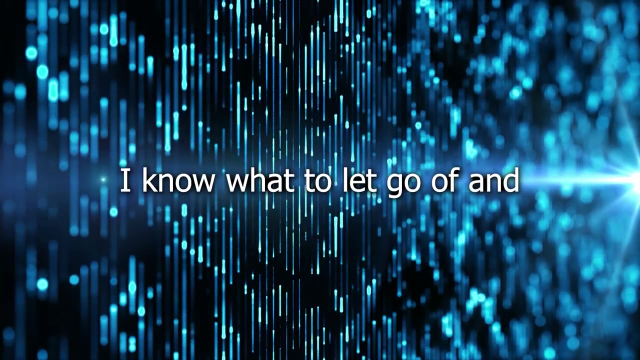 at home. I am content in the fact that I am living no longer matter. I enjoy a clear mind. Moving on comes easily to me. Ample opportunities wait for me in the future. My destiny is in my hands. Every day is a blank canvas. 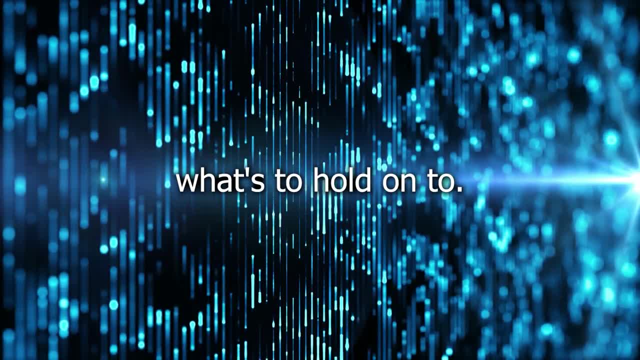 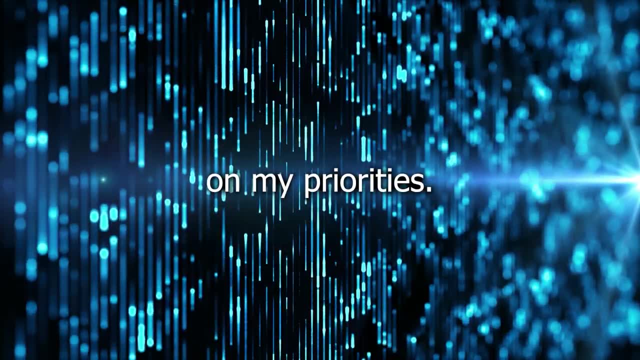 I know what to let go of and what to hold on to. Therefore, I have a blank canvas. I can identify and focus on my priorities. I am not depressedanyday. You're feeling lucky with the reflection. I am not separated from that lie. You can live. I can live and not let go of. 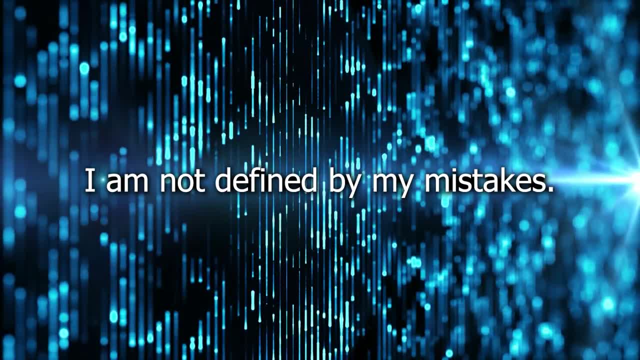 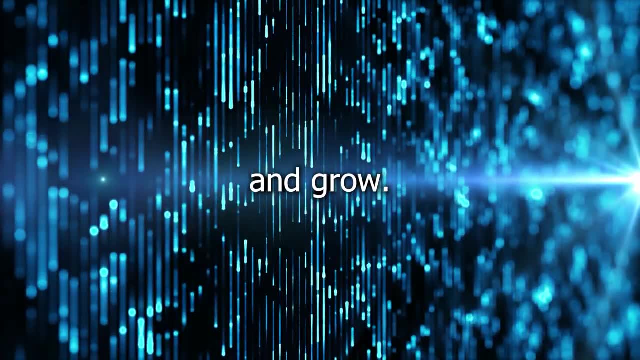 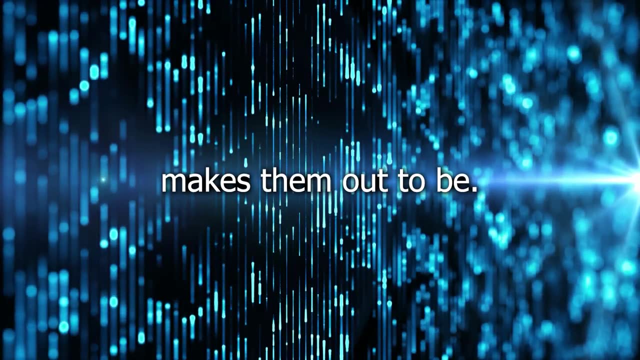 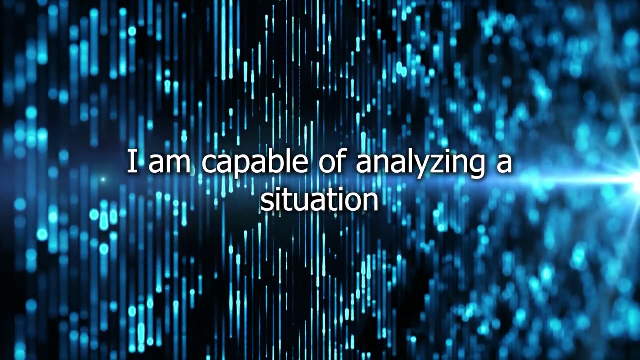 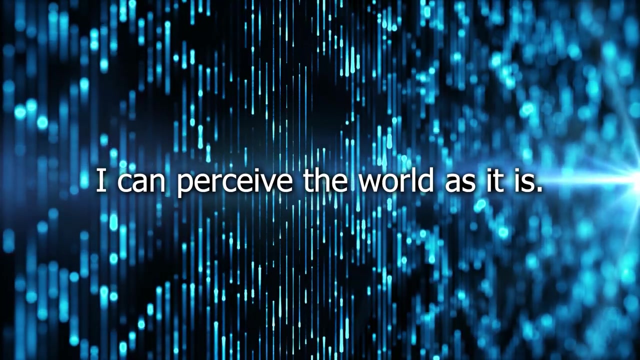 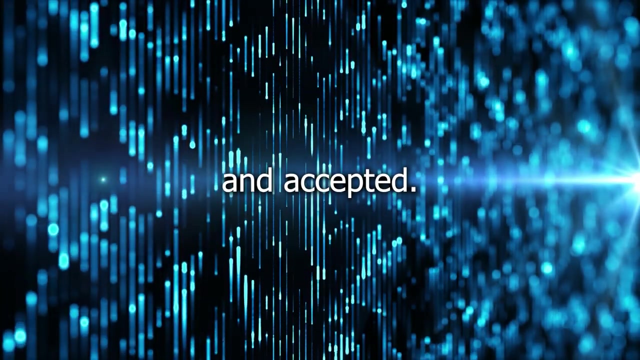 It's clear that I have returned to this village by my mistakes. Every mistake is a chance to learn and grow. Things are less scary than my mind makes them out to be. I am capable of analyzing a situation logically. I can perceive the world as it is. I am worthy of being loved and accepted. 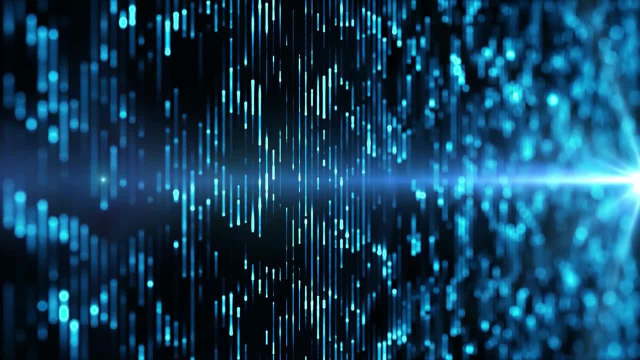 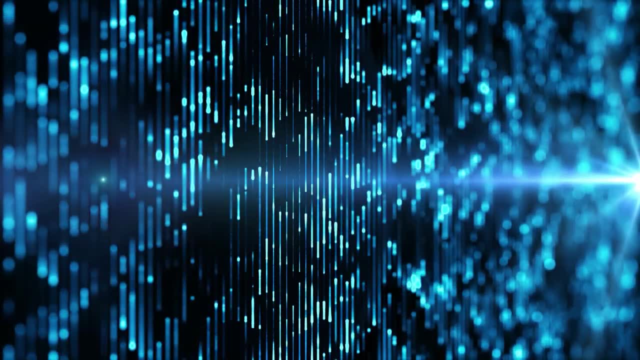 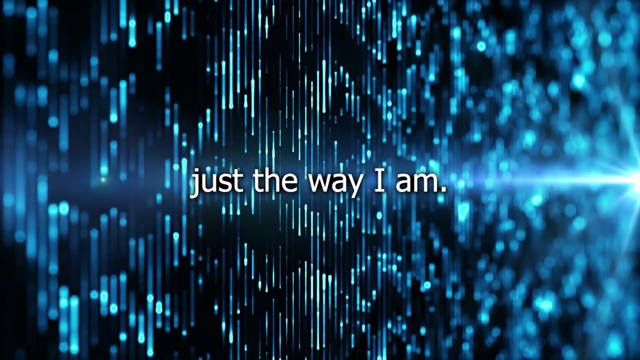 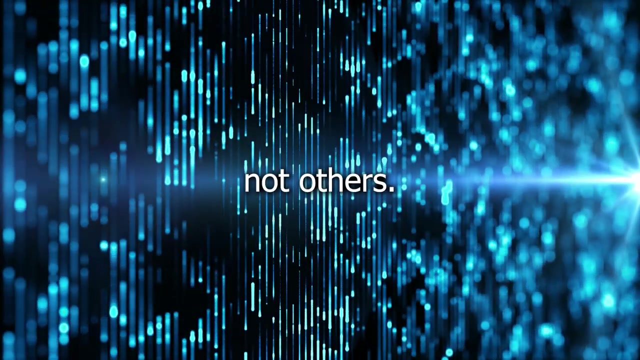 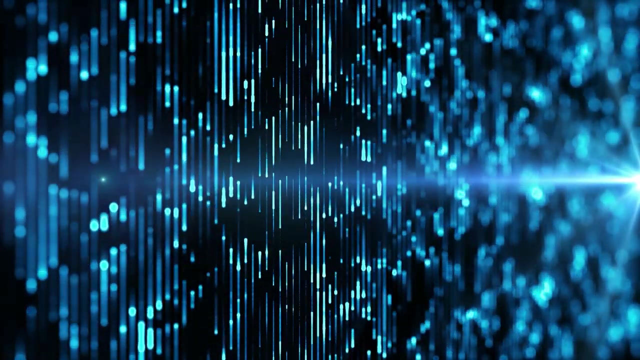 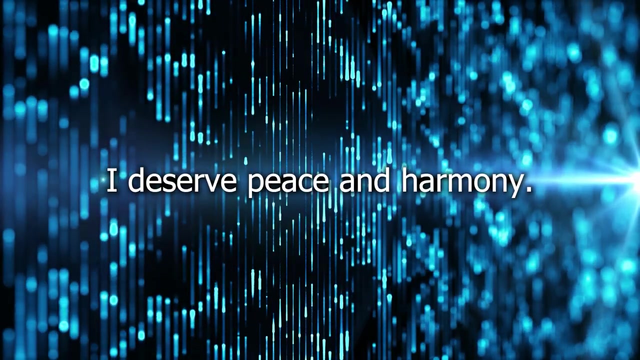 My partner loves me just the way I am. I have a partner that loves me just the way I am. I myself determine my own worth, not others. I am content with my choices and need no external validation. I deserve peace and harmony. I can remain calm and relaxed. 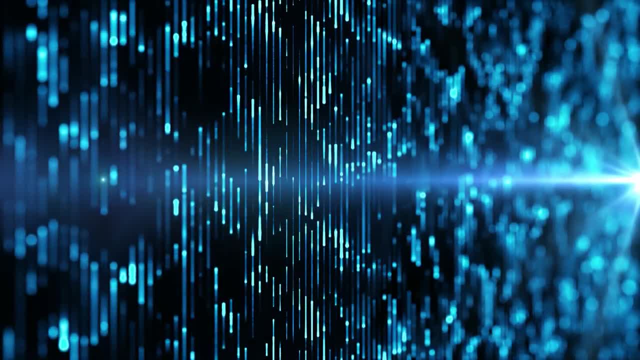 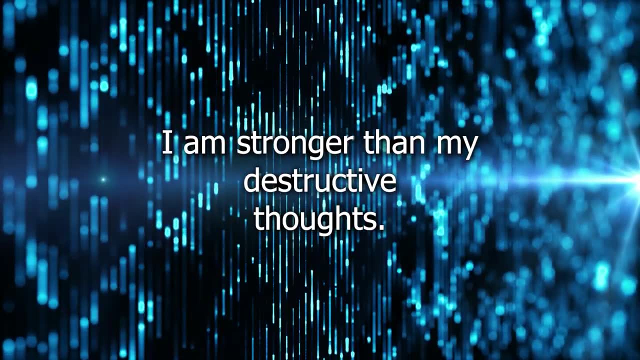 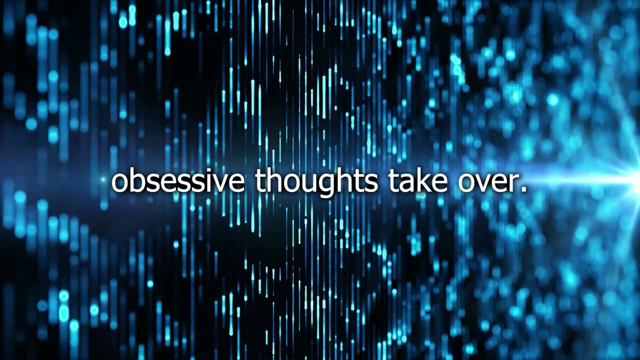 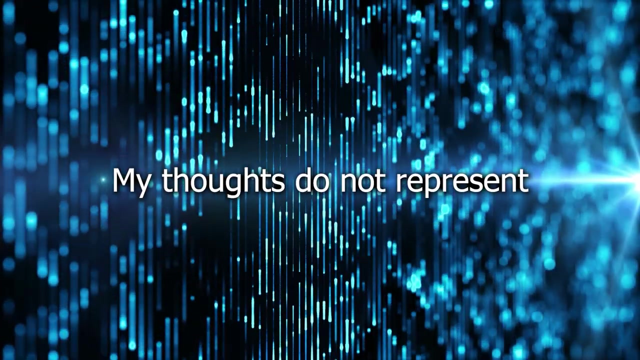 In stressful situations, I am stronger than my destructive thoughts. I refuse to let obsessive thoughts take over. My thoughts do not represent my reality. I can trust while trying to appeal to things that, in times of impoverishment, tend to mean loyalty. However, I am always being overcome by people, even people who don't believe hat. 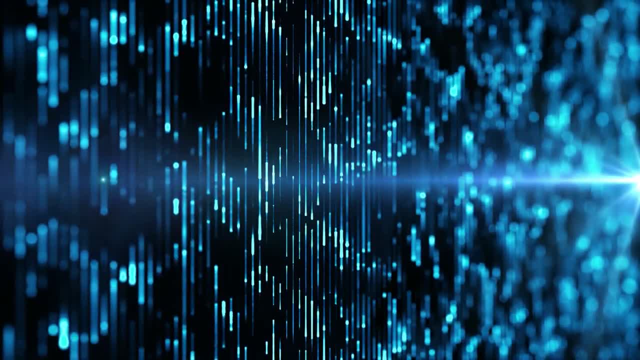 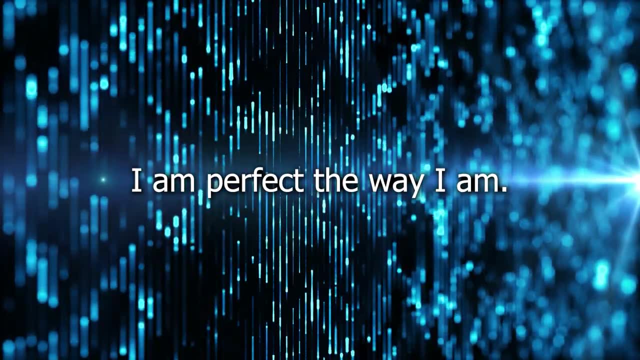 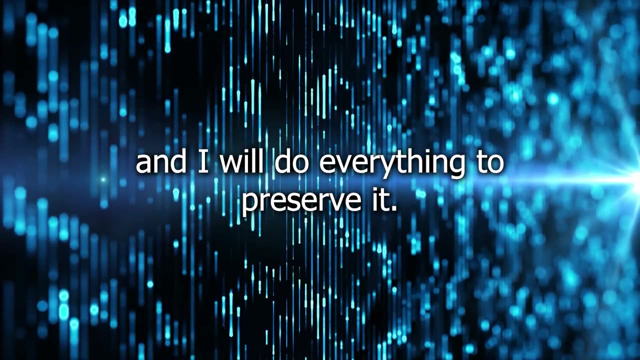 I have the ability to. I am crossing, based on myñoosh righ neighbours and myness, I can intuition. I am a kind person. I am perfect the way I am. my mental health is important and I will do everything to preserve it. I refuse to let other. 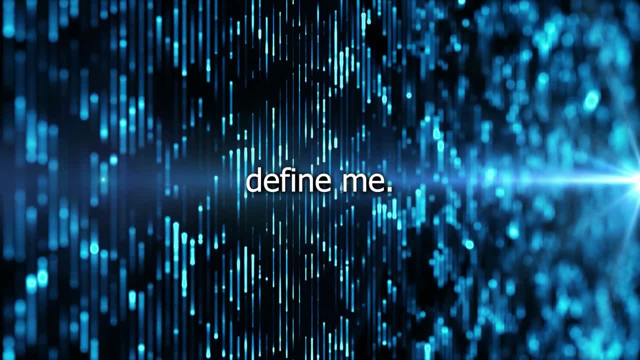 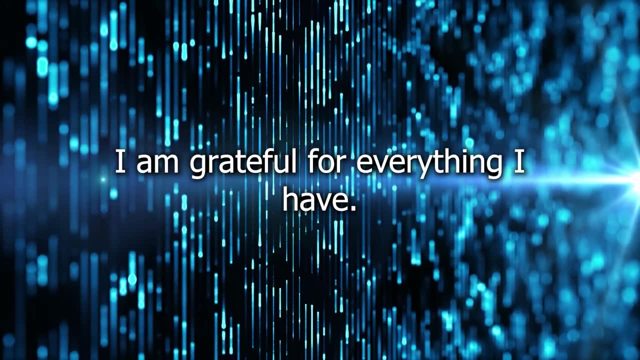 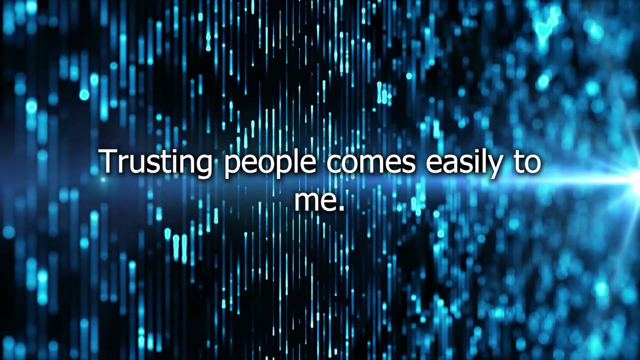 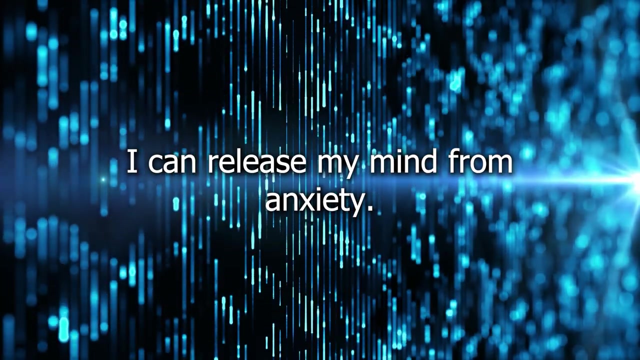 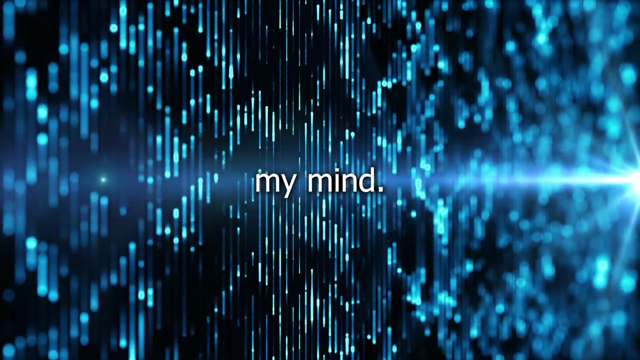 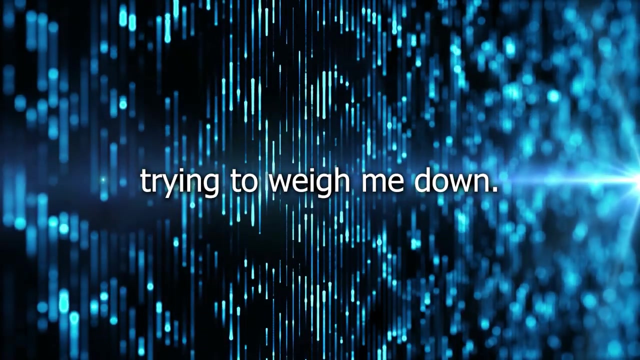 people's opinions define me. I am proud of my accomplishments. I am grateful for everything I have. trusting people comes easily to me. I can release my mind from anxiety. I am capable of decluttering my mind. I will rise above the thoughts trying to weigh me down. I refuse to.